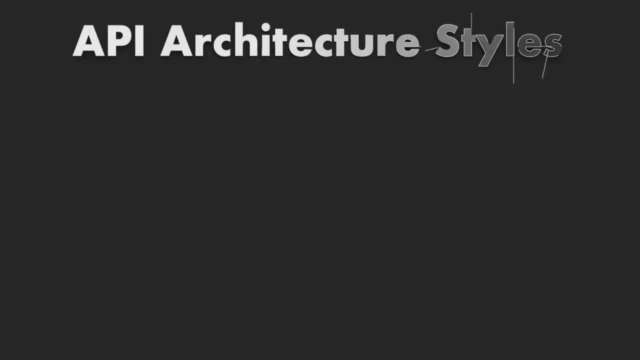 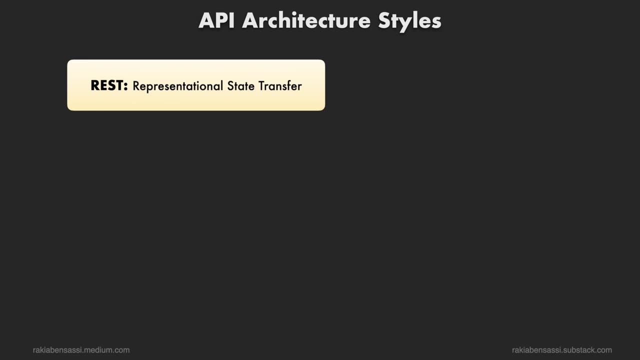 ecosystem. In the next session we'll explore the most popular styles: Rest, representational state transfer. The term representational state transfer or REST, was introduced by computer science Roy Fielding in 2000.. REST emphasizes statelessness, cacheability and the uniform interface. Its beauty lies in 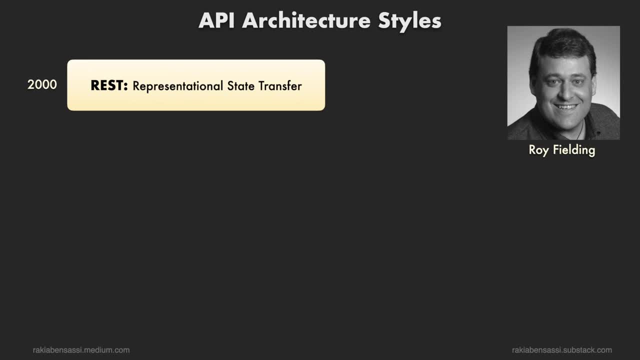 simplicity and the ability to leverage existing HTTP methods: get, post put, delete for CRUD, create, read, update, delete operations. When you browse the web, you are engaging with RESTful services, Silent yet omnipresent. The key characteristics of REST are: use of standard HTTP methods, stateless. 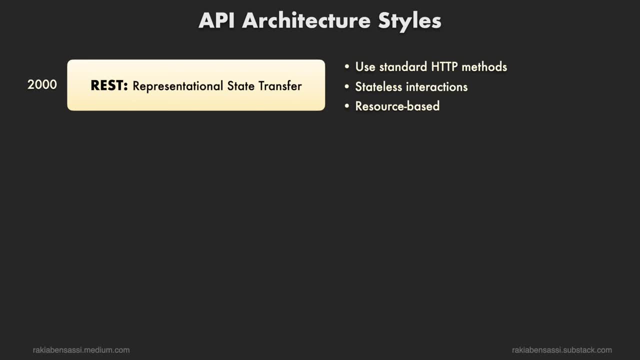 interactions and resource-based. Everything is a resource. GraphQL, a query language for your API. Next, we have GraphQL, which is a query language for your API. It was released as open source by Facebook in 2015 and presents a revolutionary way to fetch data. 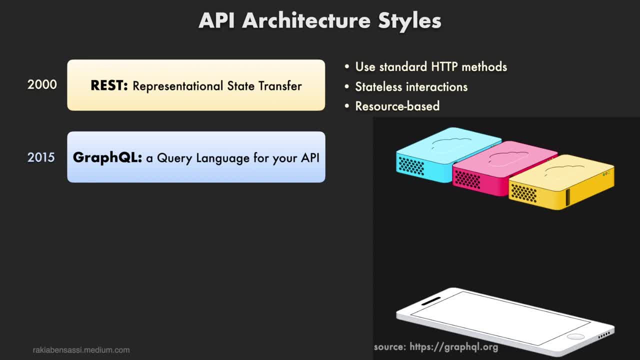 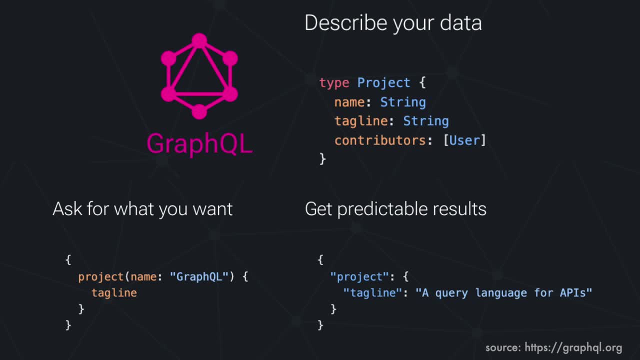 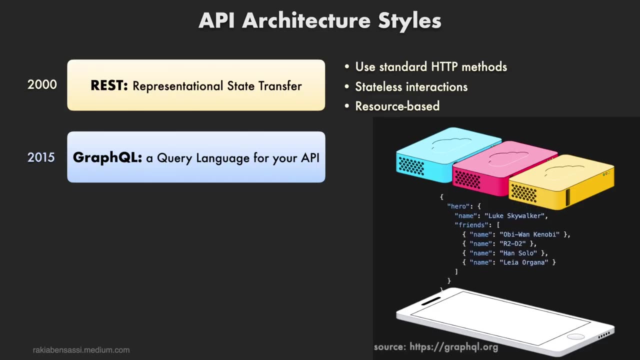 Unlike REST, where you may need multiple requests to gather various pieces of information, GraphQL lets clients specify exactly what they need in a single query. It's like having a conversation with your data, asking what you want and getting precisely that. no more, no less. 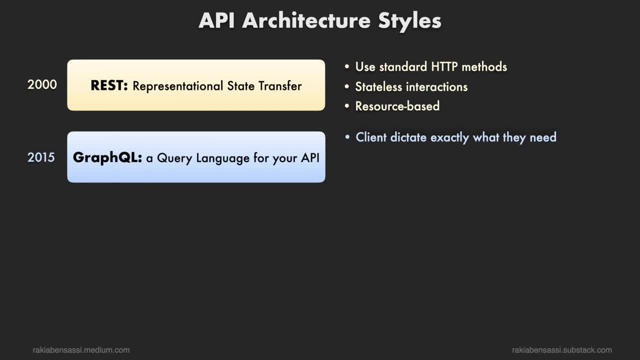 The key characteristics of GraphQL are: Clients dictate exactly what data they need. It allows fetching data from multiple resources. Kindly note: it affects teams, network servers, house settings, execution and Inspectoryou can repeat the task of each of these tasks from months to months, But GraphQL can、. 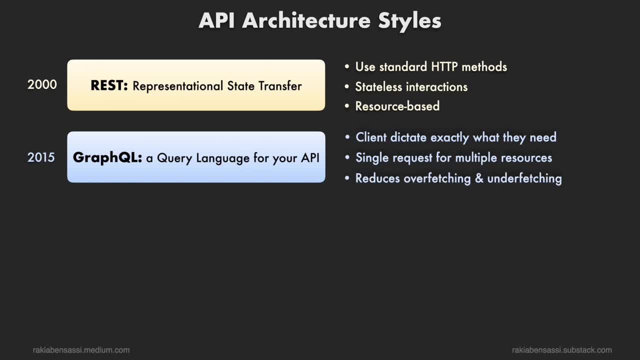 help nurses to develop their mode of working the structure of the team. experienceREST can reduce communication processes in a single request And it reduces overfetching and underfetching, which are common issues in REST APIs. SOAP, Simple Object Access Protocol. 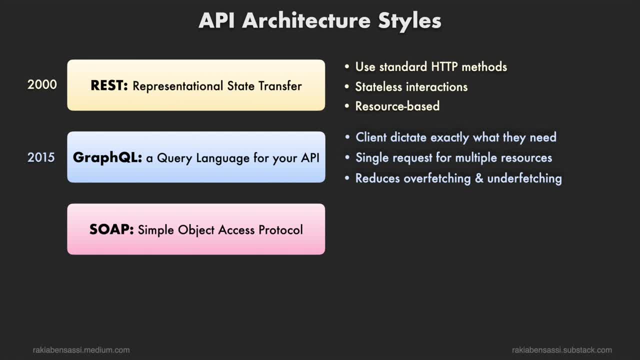 SOAP was designed as an object access protocol and released as XML RPC in 1998.. It's the elder statesman of web services, heavily favored in enterprise environments for its strict standards and security features. With SOAP, everything is enveloped in XML, which offers high level of formal contracts. 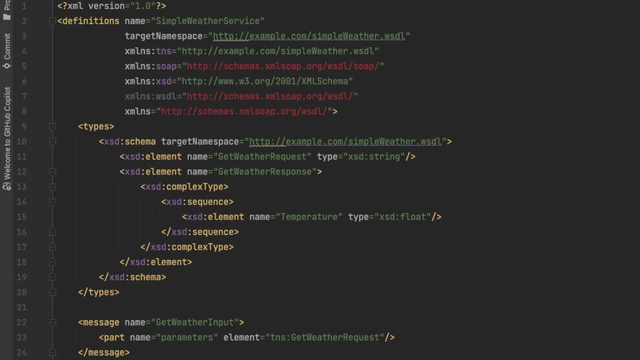 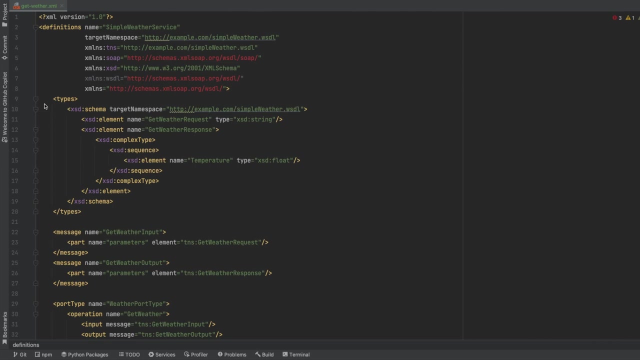 via WSDL or Web Services Description Language documents. It's like sending a certified letter, more formal, with a clear understanding of the contents and delivery expectations. Here is an example of a SOAP WSDL file for a weather service. It provides the GetWeather operation for getting the current weather based on a city name. 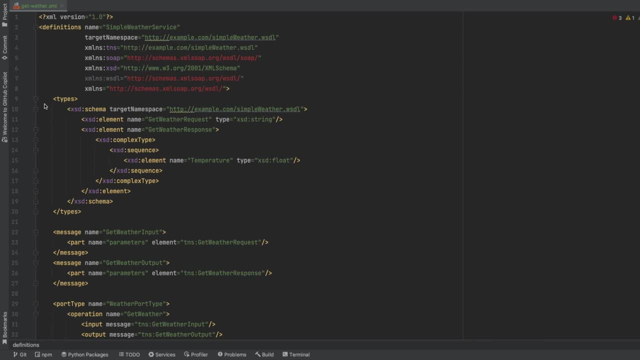 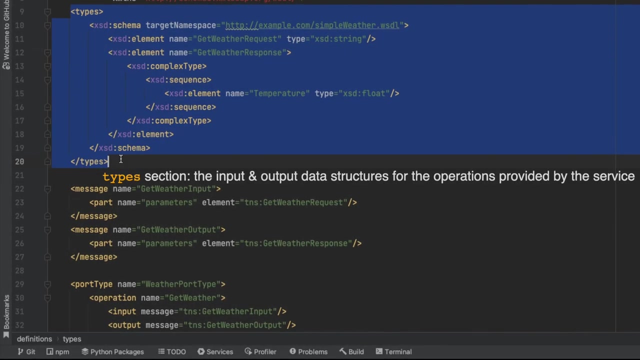 It provides a machine-readable description of how the weather service can be called, what parameters it expects and what data structures it returns. It's a way for clients to understand how to interact with the service without knowing the underlying implementation details. In this WSDL document, the Types section defines the input and output data structures for the. 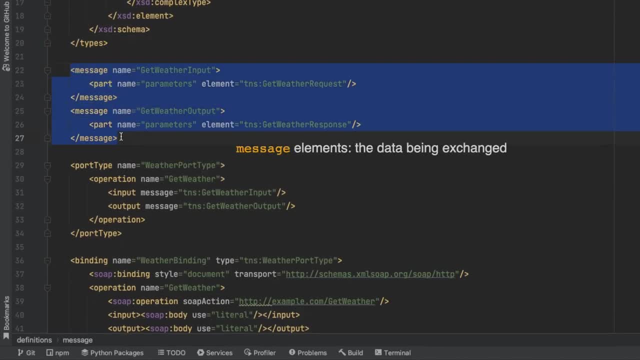 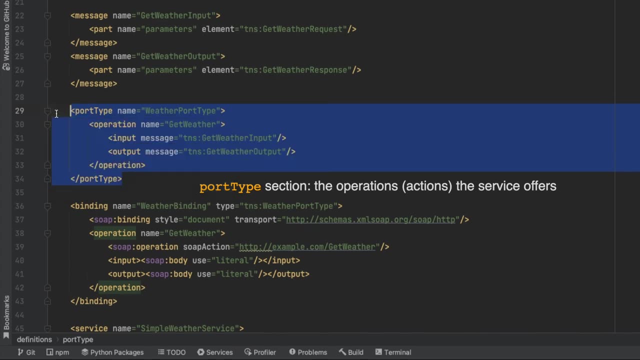 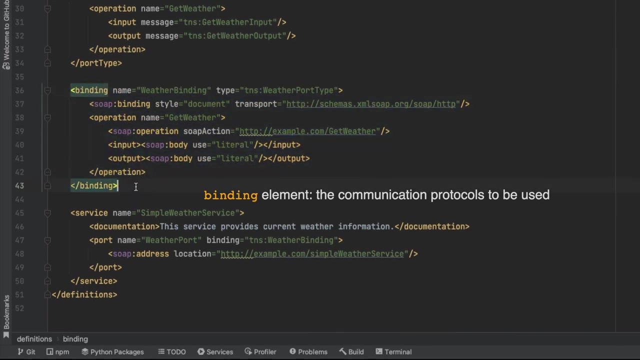 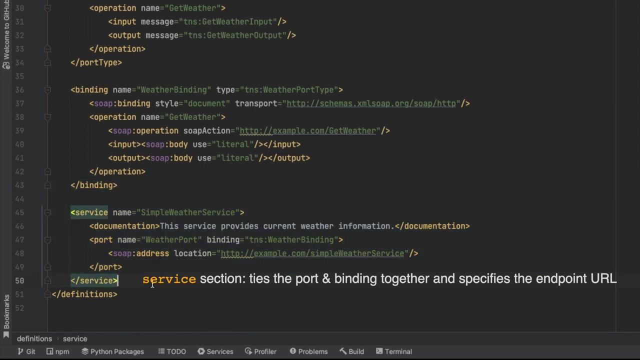 operations provided by the service. The message elements define the data being exchanged. The port type section defines the operations or actions the service offers. The binding element specifies the communication protocols to be used. Finally, the service section ties the port and binding together and specifies the endpoint. 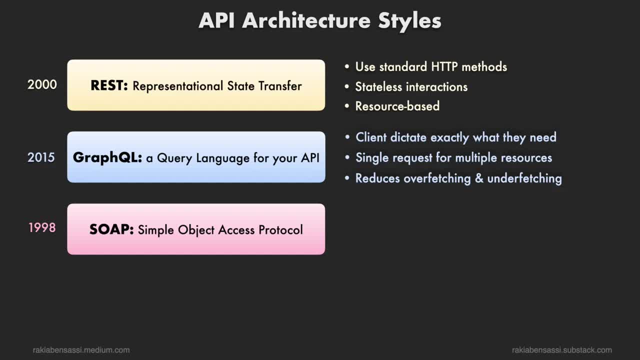 URL. The key characteristics of SOAP are protocol agnostic, It can work over HTTP, It can work over IP address, It can work over IP address, It can work over HTTP, SMTP, TCP, Strongly typed operations, and it emphasizes on security and transaction compliance. 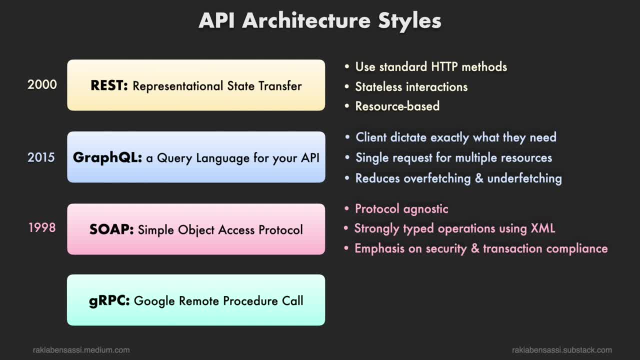 GRPC was developed by Google and released as open source in 2016.. The new Gradient cycle was added as the distance is kept on the startup network, It is virtually on-. juegos. Taylor Hayes, Kibleszdl and the Generator: Media transformation. 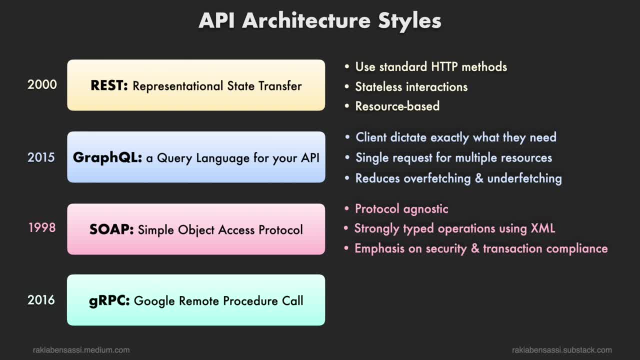 pegato. Its functions are rigorous. They can be ig specialists and numerous Rêtes expressions can use 7-bit code traffic. To differentiate the data didn't need an IP address and a server. A node can template everything about the data. 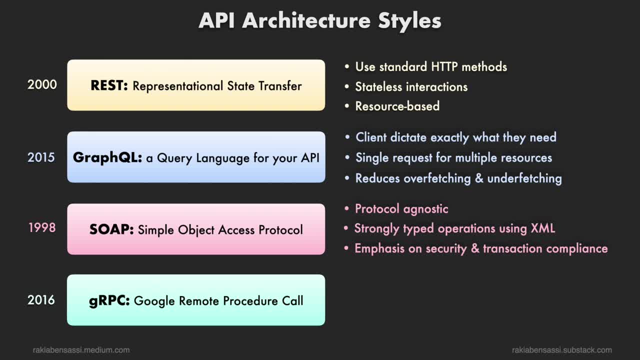 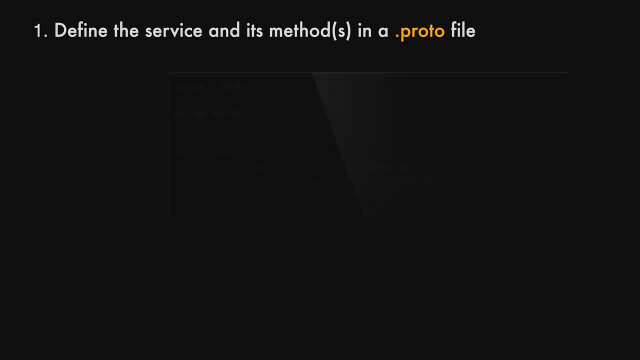 port protocol buffers as the interface description language and provides features such as authentication, load balancing and more. it's akin to having a private express lane for your data, ensuring fast and efficient communication. here is how to define the get weather service and its method in a protobuf file. this file acts like the contract between the server and the client. 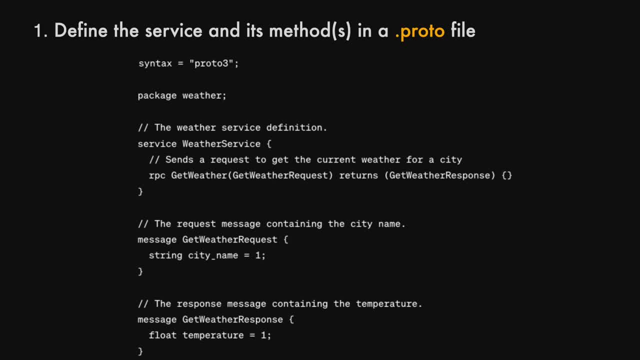 it defines the structure of the request and response messages. in this example, we define a weather service with a method: get weather. this method takes a get weather request message containing ct name and returns a get weather response message containing the temperature. we can call the specified method remotely with its parameter and return type, once the dot. 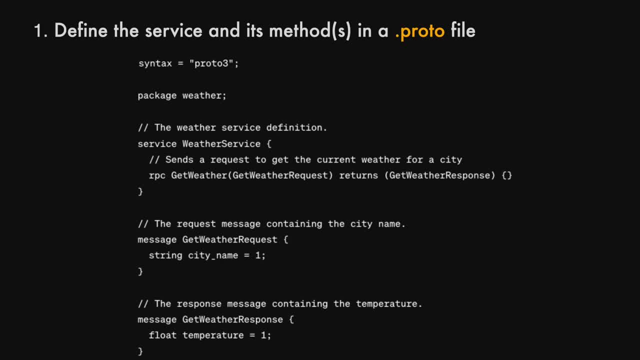 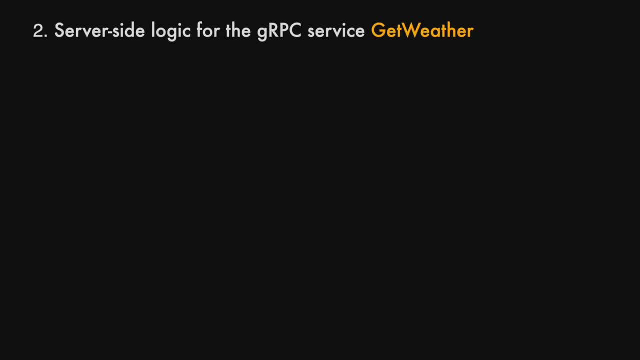 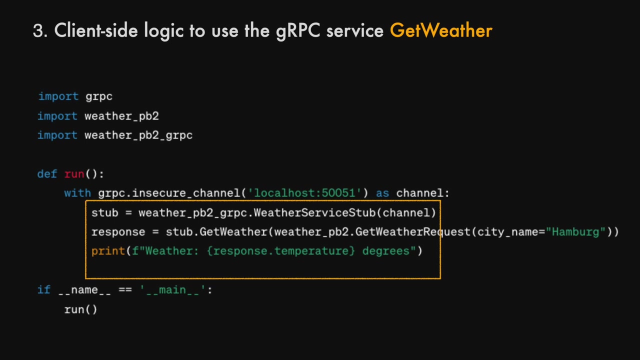 proto file is defined, the protocol buffers compiler generates client and server code in your chosen language. Then you can implement the server-side logic, like in this code snippet where you specify the logic to fetch the weather inside the getWeather method. The following code snippet shows the client-side logic. It sends a request to the server and prints out the temperature it. 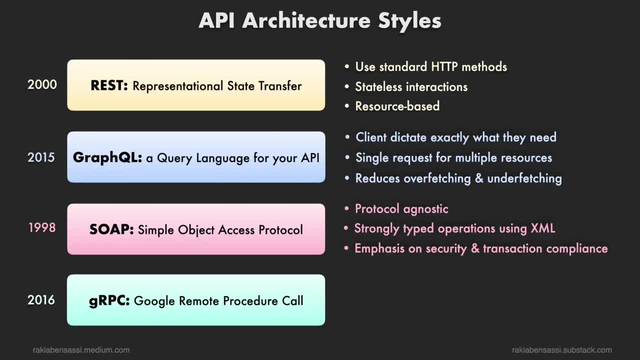 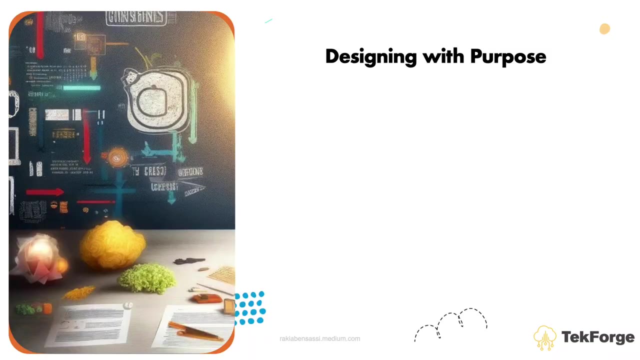 receives in the response. The key characteristics of gRPC are: use of HTTP2 for lower latency and better compression. use of protocol buffers or protobuf, which provides a more efficient and compact serialization format, and it supports streaming requests and responses. Designing with purpose. In order to choose the appropriate architectural style, you need to consider your 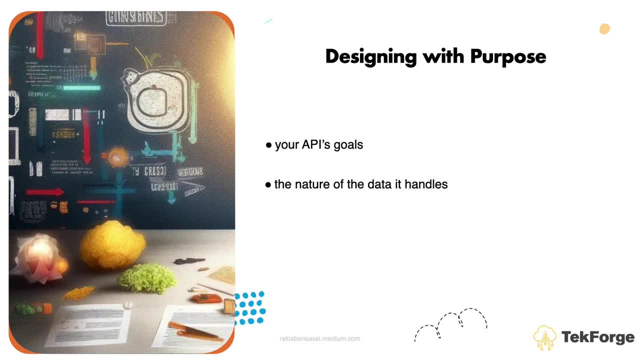 API's goal, the nature of the data it handles and how it will be consumed. There is no one-size-fits-all answer here. The best choice is to use gRPC. Are you building a public-facing API with a broad consumption? In this case, REST or GraphQL might. 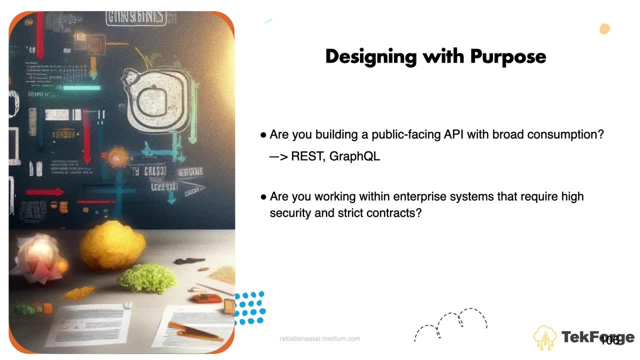 be your best bet. Are you working with enterprise systems that require high security and strict contracts? Then SOAP could be the way to go. Do you need high performance and efficient communication for microservices? Take a closer look at gRPC Hands-on challenge. 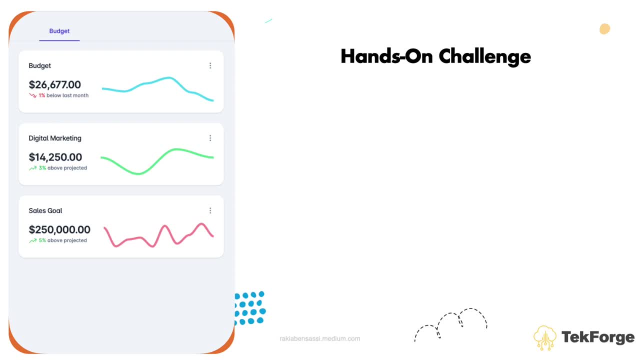 Let's put theory into practice now. Imagine you are designing an API for a mobile app that requires real-time data updates and efficient communication. Which architectural style would you choose and why Consider the app's need, data complexity and the user experience you aim to? 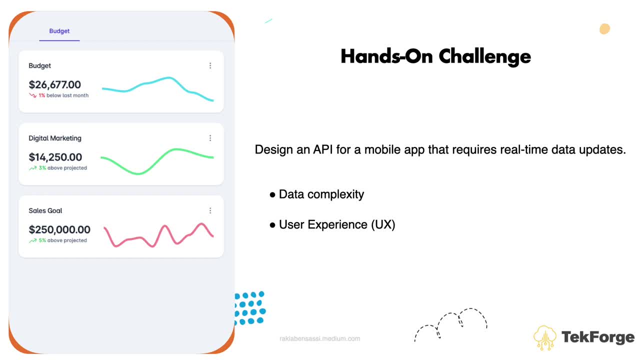 provide. As we wrap up this section, remember that the art of API design lies not just in understanding these styles, but in knowing what they are, When and how to apply them effectively. Embrace these architectural philosophies as you continue to sculpt your APIs, and you will find yourself not just building APIs, but crafting experiences. 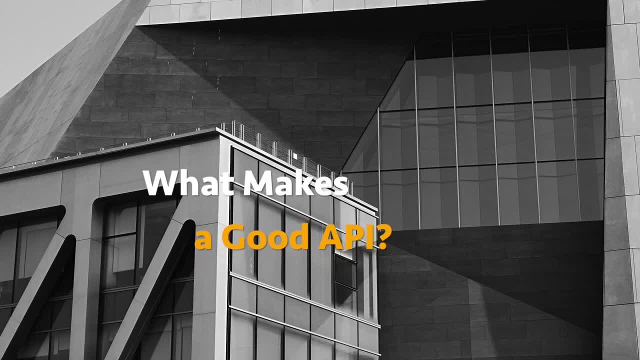 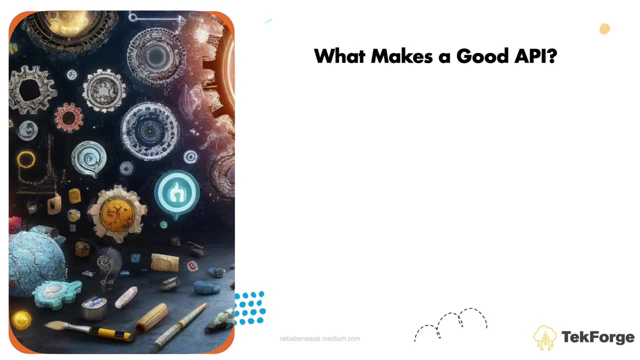 that enrich the digital world. What makes a good API? The landscape of API architecture is rich and varied, offering a toolbox of options to tailor your API's design to its intended purpose and audience. So what makes a good API? First, we have simplicity and intuitiveness. A good API is easy to understand and use. 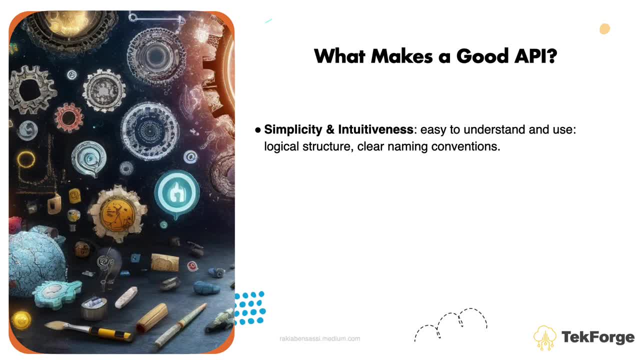 even for developers not familiar with the underlying system. It should have a logical structure, clear naming conventions and be as intuitive as a well-designed user interface. Consistency in API design promotes easier learning and understanding. This means consistent naming, request-response format and error handling across your API. 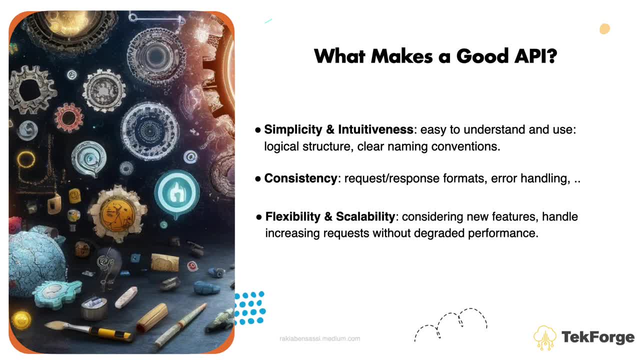 Flexibility and scalability. APIs should be designed with future growth in mind. This includes considering how new features can be added or how the API can handle increased loads or requests without degraded performance. Security- An often overlooked aspect, yet vital, is the security of your API. 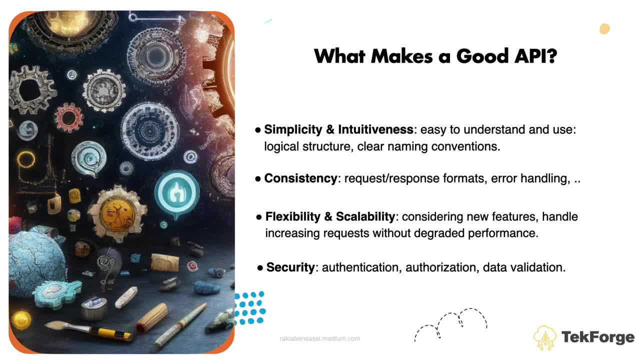 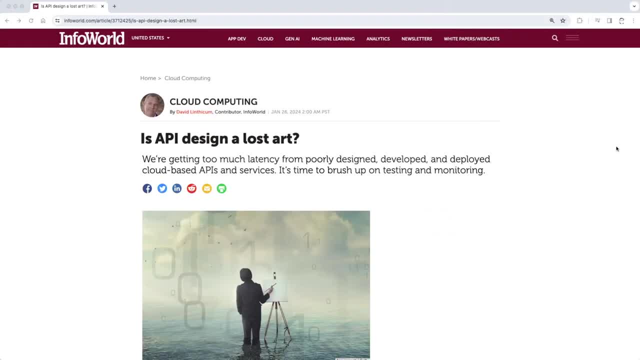 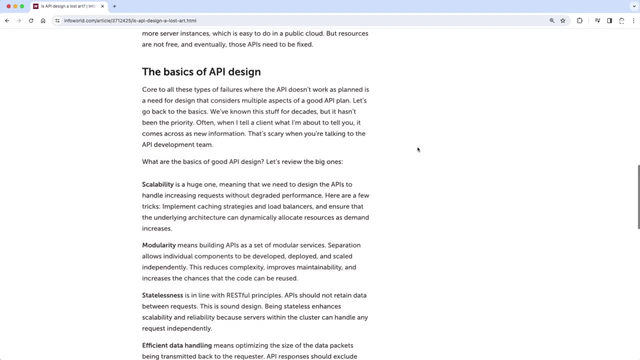 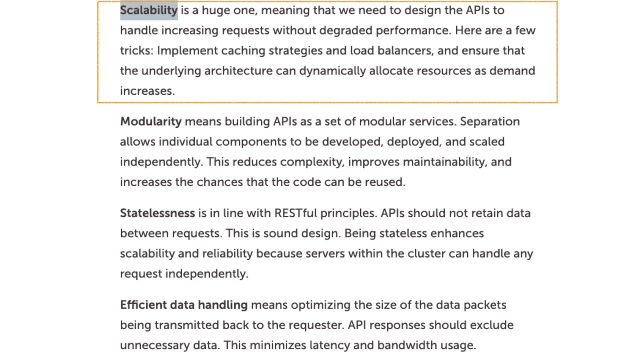 Implementing authentication, authorization and data validation are key to protecting your API from misuse. In his very insightful article on InfoWord: Is API Design a Lost Art? David Linficom highlighted four basics of good API design, which are: Scalability, As I already mentioned, APIs need to handle increasing requests without degraded performance. 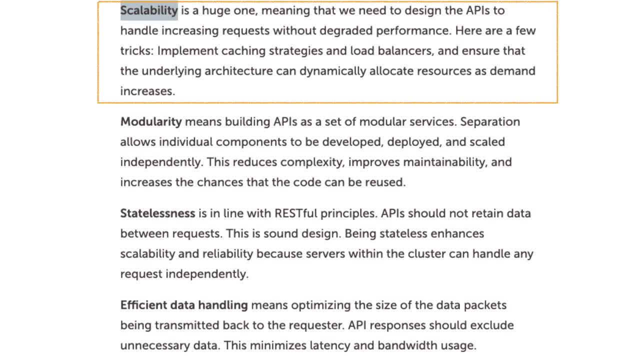 For that sake, we can leverage caching strategies and load balancers and ensure that the underlying architecture can dynamically allocate resources as demand increases. Modularity: Building APIs as a set of modular services offers a separation that allows individual components to be developed, deployed and scaled independently. 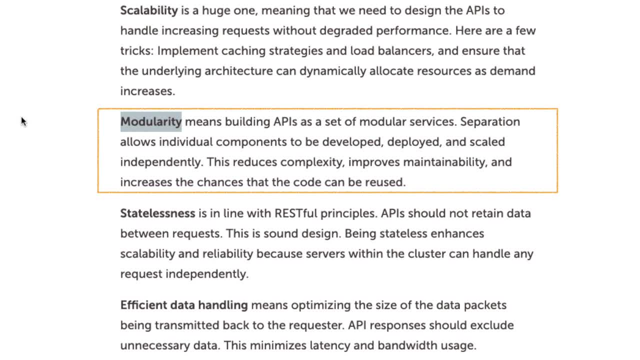 This increases the code reusability, improves maintainability and reduces complexity. Statelessness, Which is part of the code Stability- The restful principles. APIs should not retain data between requests. This way, servers within the cluster can handle any request independently. 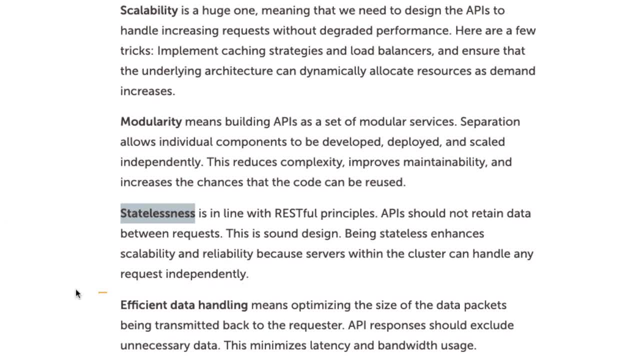 which enhances scalability and reliability. Efficient Data Handling API responses should exclude unnecessary data in order to optimize the size of the data packets being transmitted back to the requester. This minimizes latency and bandwidth usage. Real-world applications: Let's dive into an example now. 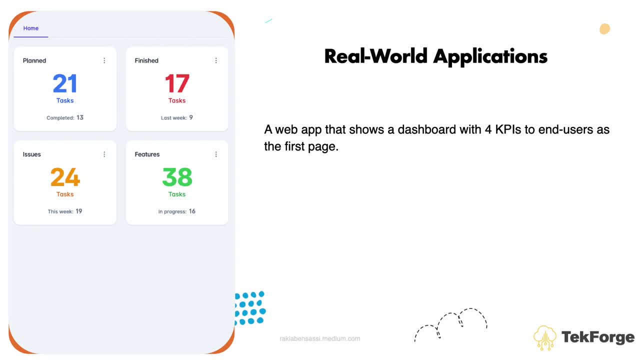 Consider a web app that shows a dashboard with four KPIs, or key performance indicators, to end users as the first page whenever they call it. That web app retrieves the values for these KPIs from a REST API by sending four HTTP requests. 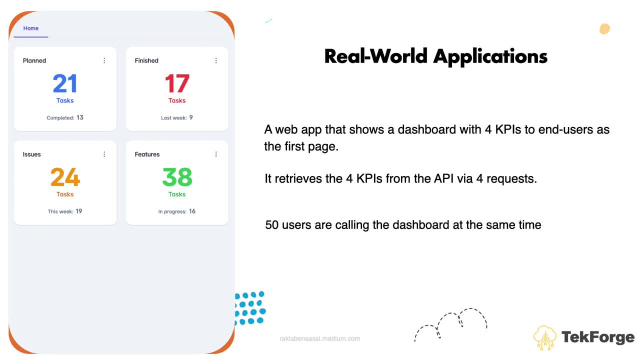 Let's imagine now that 50 users are all calling the dashboard page at the same time. This means the REST API will receive 200 requests just to deliver the KPIs data to the end clients. If all the four KPIs' values could be delivered in a single request instead of four. 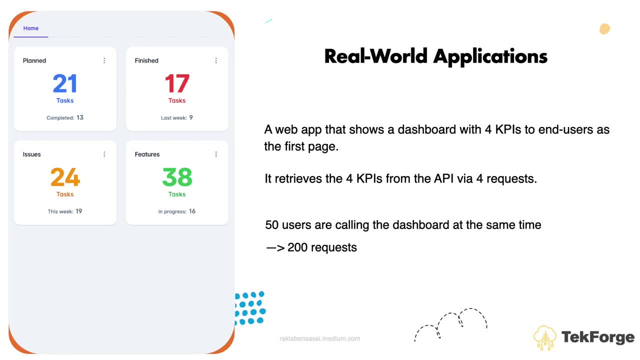 the REST API will handle only 50 requests for the 50 users. What do you think about this scenario? Is the implementation of one request per KPI correct or wrong? Well, the right answer is: it depends. It depends because there are many factors that we need to consider. 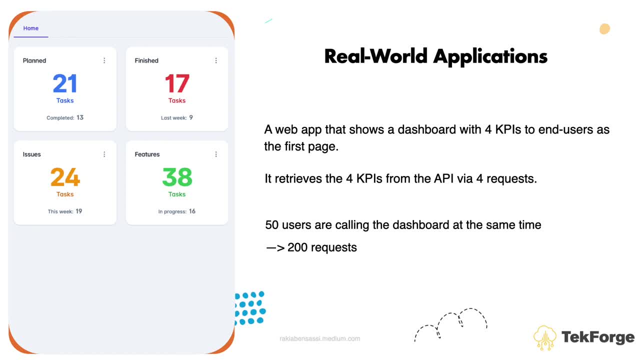 in order to opt for a better approach to our API design. Let's have a look at these factors: Flexibility: Multiple calls offer more flexibility and allows the client to request only the data it needs at any given time. Yet if you don't have different parts of the application, 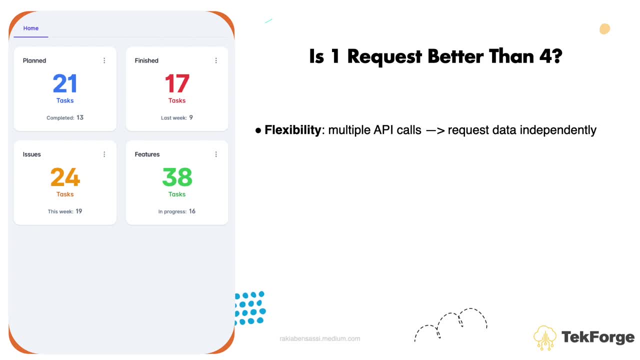 that need to display different KPIs independently. it might be better to use just one call for the dashboard data Performance. A single API call reduces the overhead of establishing multiple TCP connections and the round-trip time for each request. Thus it can be faster than multiple calls. 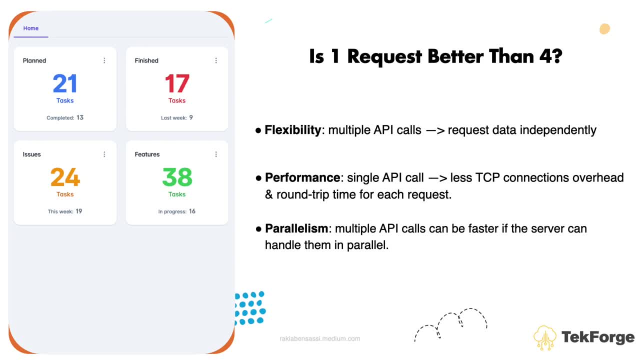 Parallelism. In some cases, making multiple calls can be faster if the server can handle them in parallel. But let's say that you have a REST API implemented with the Django Python framework. In this case you need to consider the following: Django by default is single-threaded: one request at a time. 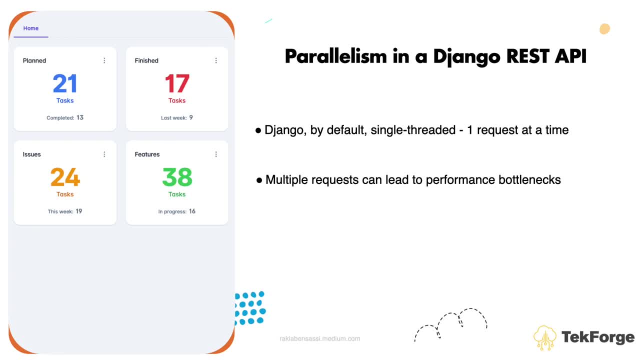 This can lead to performance bottlenecks when handling multiple requests concurrently, especially when the server is under heavy load. To handle multiple requests in parallel in a Django application, you can use a WSGI server that supports concurrency better, such as Junicorn. 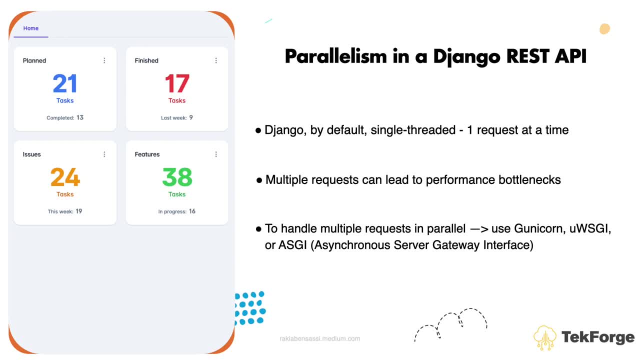 UWSGI or ASGI, a synchronous server-gateway interface. Now, if you want to use a single-threaded application, you need to consider the following: If you switch gears and look at a REST API built with Java, specifically using Spring Boot, the parallelism story changes a bit. 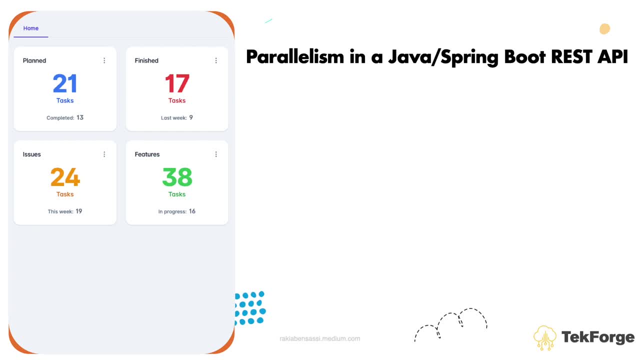 Spring Boot apps are a whole different beast. Java's ecosystem, including Spring Boot, inherently supports multithreading, making it easier to handle multiple requests at once, right out of the gate. Spring Boot's concurrency model lets you handle tons of requests simultaneously without breaking a sweat. 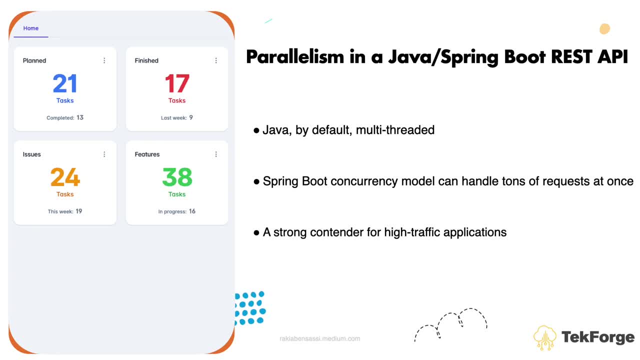 It's built to juggle, making it a strong contender for high-traffic applications. Plus, with the right setup, Spring Boot can scale up to manage even more parallel requests thanks to Java's robust threading and concurrency support. So, while Django needs a bit of a push, with a compatible server to handle the crowd. 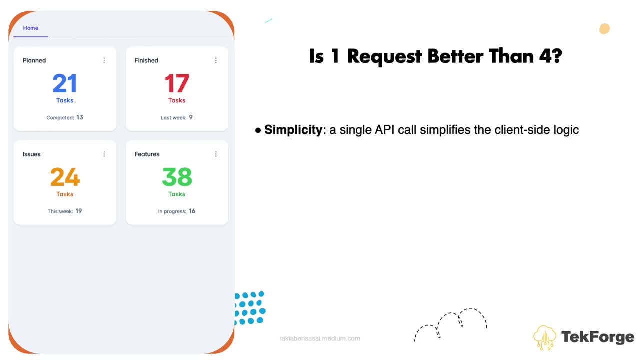 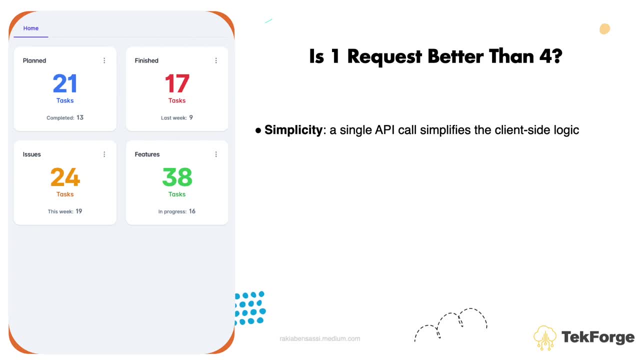 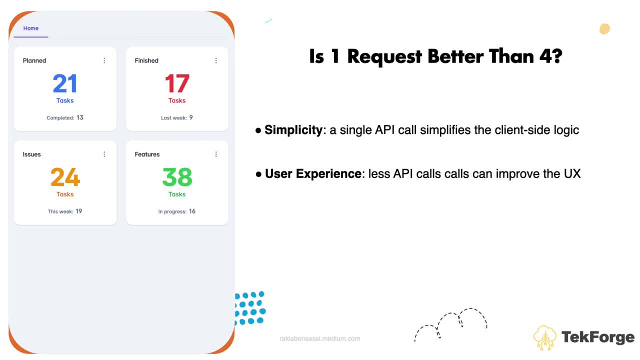 User experience For mobile apps. minimizing the number of calls can improve the user experience. Caching A single call allows for more efficient caching strategies. The server can cache the responses for a short period, which reduces the load on the server and improves response times for subsequent requests. 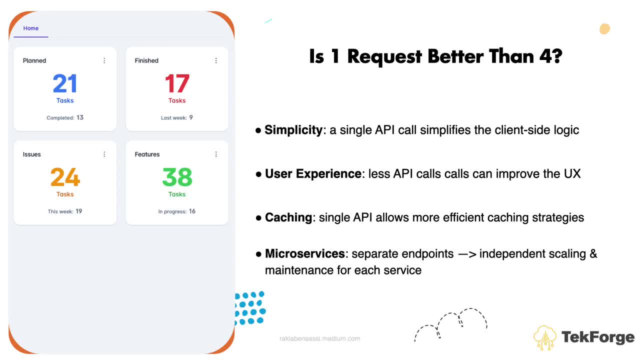 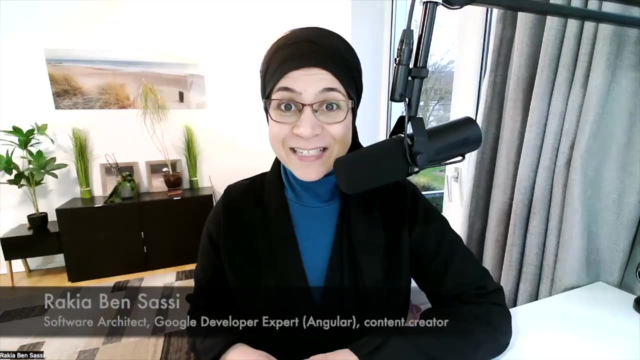 Microservices architecture. If your system follows a microservice architecture, having separate endpoints for each KPI might align better with the server-oriented design. It allows for independent scaling and maintenance of each service. Excited about diving deeper into the world of software architecture?